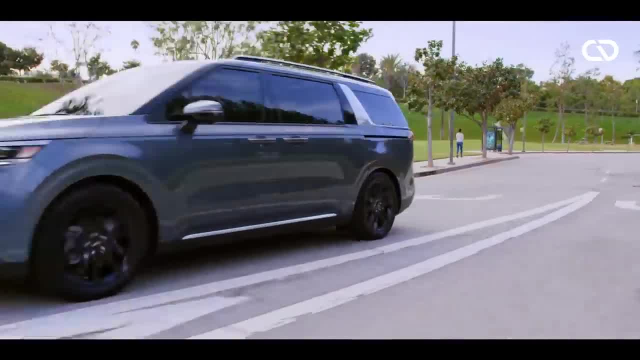 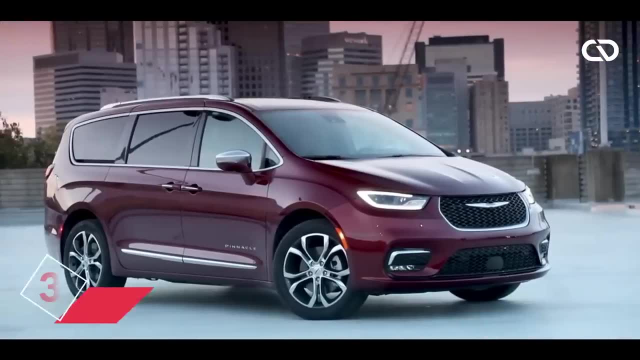 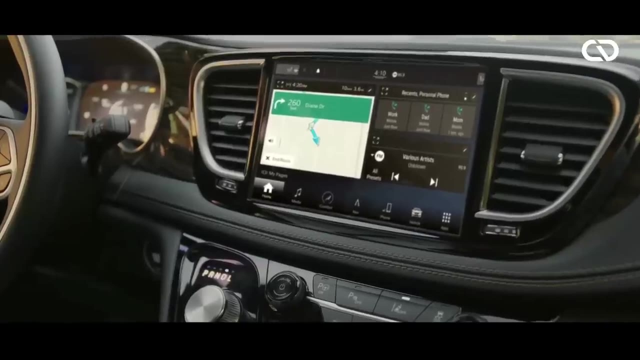 efficient and all-wheel drive, which is very important on a large-size vehicle, then another minivan on our list might be perfect for you, which is the 2023 Chrysler Pacifica. The 2023 Chrysler Pacifica is the perfect choice for families on the go, With spacious seating in. 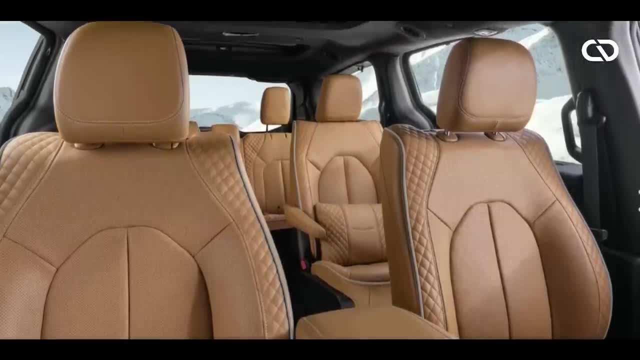 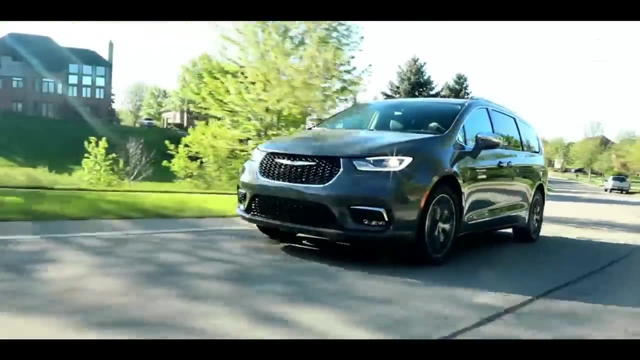 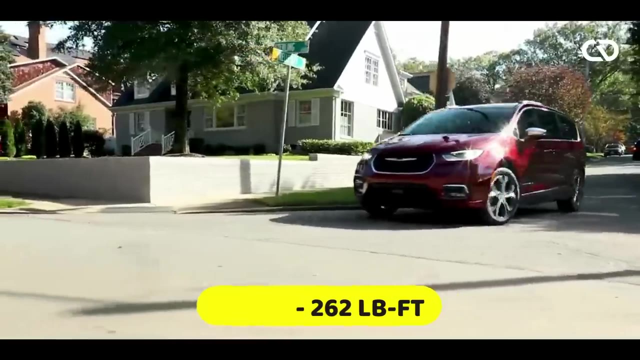 all three rows, ample cargo space and a host of standard features. the Chrysler Pacifica offers everything you need for comfortable and convenient travel. All Pacifica comes equipped with a simple 3.6-liter V6 that makes 287 horsepower and 262 pound-feet of torque. 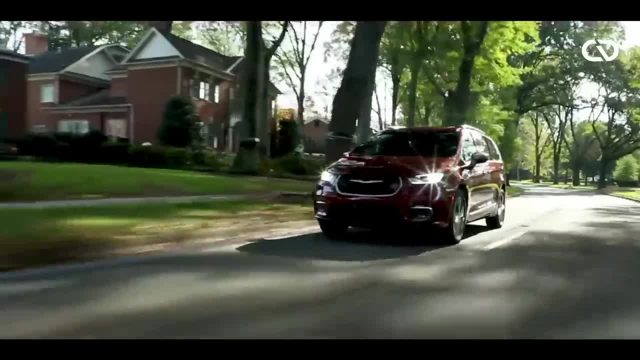 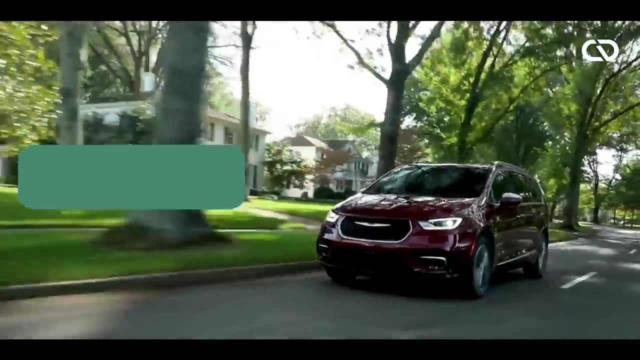 Front-wheel drive is standard, while all-wheel drive can be added for a few extra dollars, And the Pacifica is the only minivan that offers plug-in hybrid powertrain options, featuring the same 3.6-liter V6, along with two electric motors and a 16-kilowatt-hour battery pack. 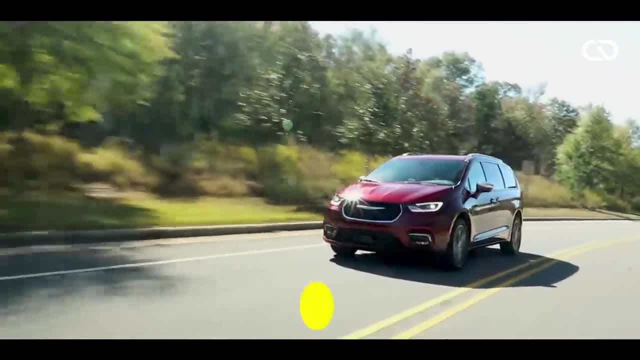 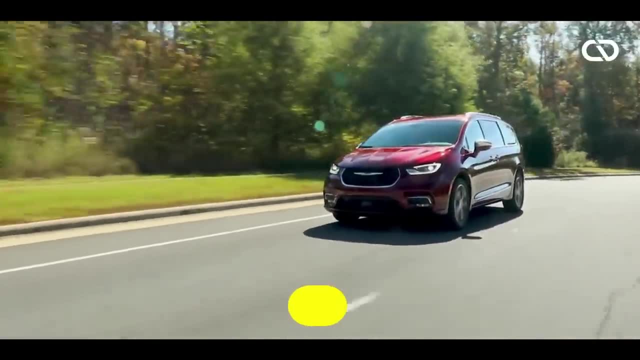 This means that you will get 84 mpge combined and an impressive 33 miles of pure electric range as well. Although the plug-in hybrid variants come with a somewhat high starting MSRP, which we don't recommend to our viewers, we highly recommend the mid-range Touring L trim. 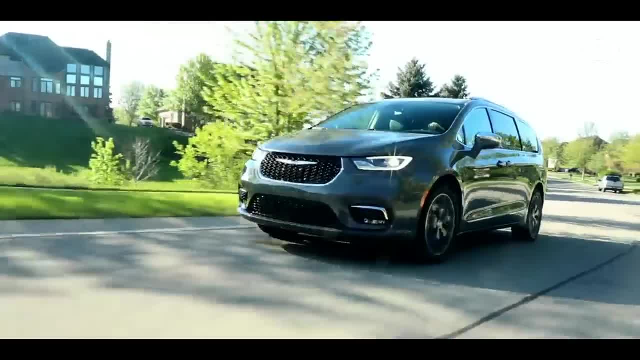 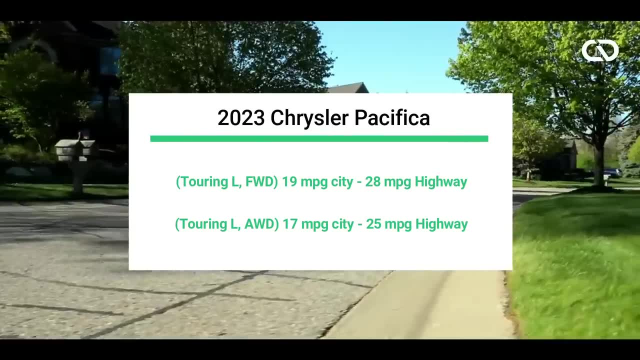 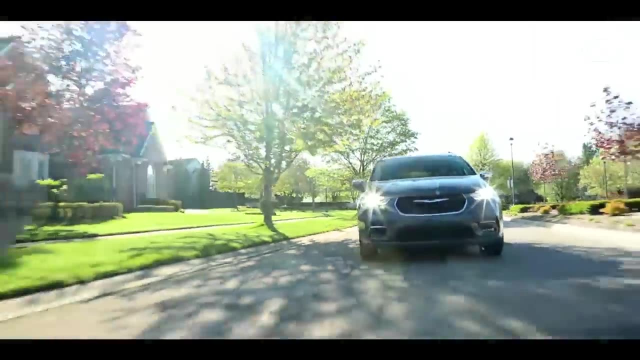 as the best value for the money, and it offers plenty of additional features over the base model. Additionally, the Touring L front-wheel drive variant has a fuel economy of 19 miles per gallon in the city, miles per gallon on the highway. When it comes to the towing capacity, well, the Pacifica can. 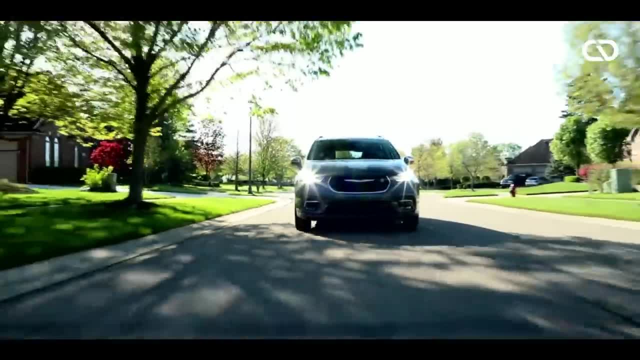 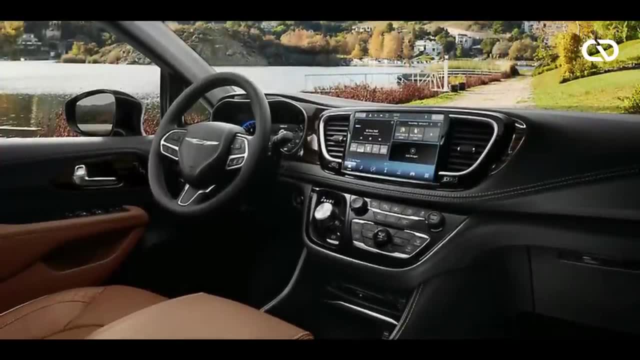 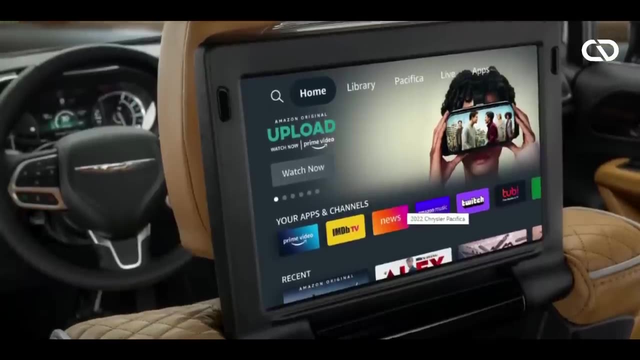 tow up to 3,600 pounds, which is about 100 pounds more capacity than the Kia Carnival. The interior is well-designed. The minimalist dashboard comes standard with a 10.1-inch touchscreen with Android Auto and Apple CarPlay and a 7.0-inch driver display. Also the Pacifica. 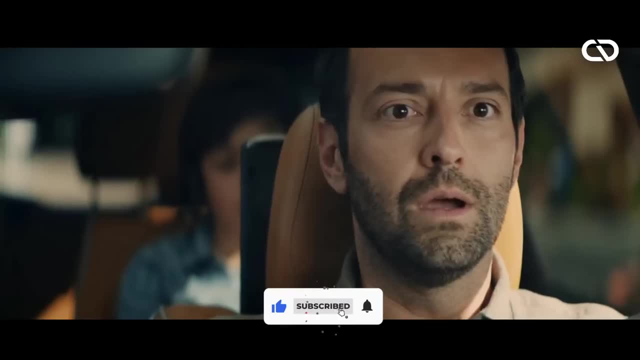 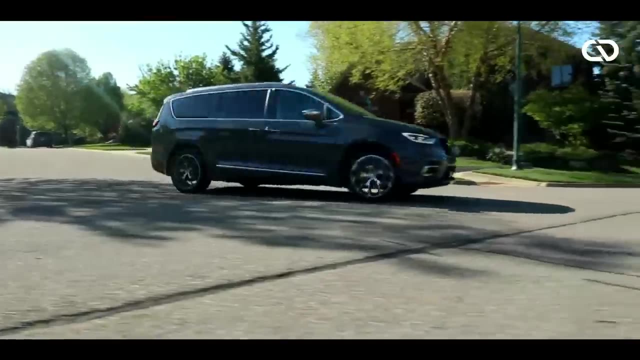 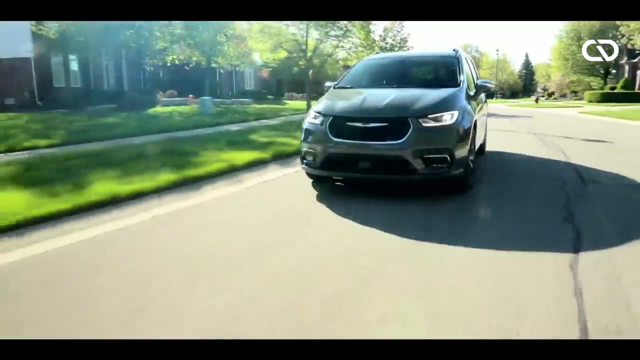 comes standard with a lengthy list of safety features, including automatic emergency braking, blind-spot monitoring and adaptive cruise control. Despite the Pacifica having a poor predicted reliability score and the base trim starting at somewhat high MSRP, if you're looking for something reliable and cheaper, then let's check out the number two vehicle on our list. 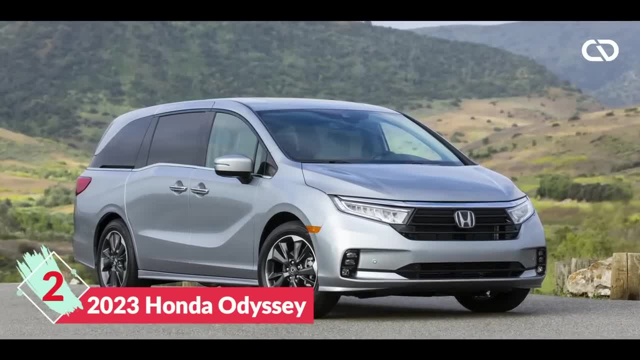 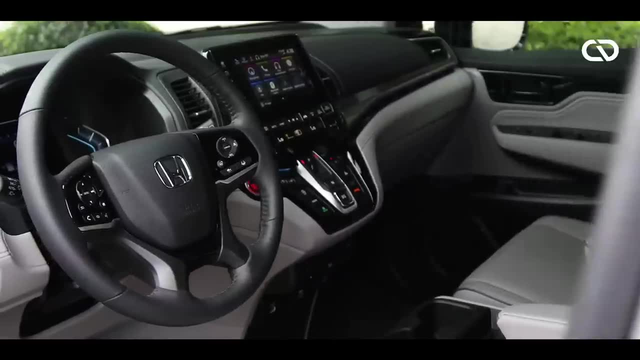 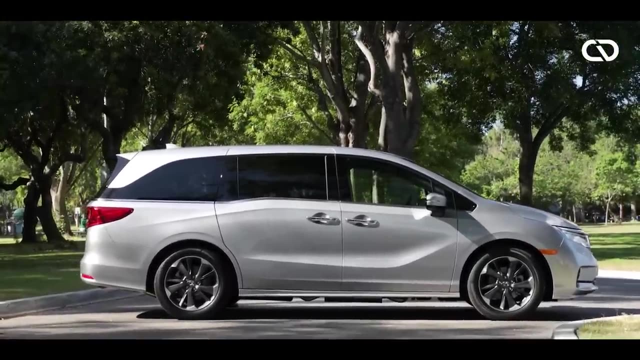 Which is the 2023 Honda Odyssey. If you're looking for long-term reliability, better performance, strong build quality and practicality in a minivan, then the 2023 Honda Odyssey is worth considering. Under the hood, the Odyssey has a very reliable engine, which is a naturally aspirated 3.5-liter V6.. Not only is this 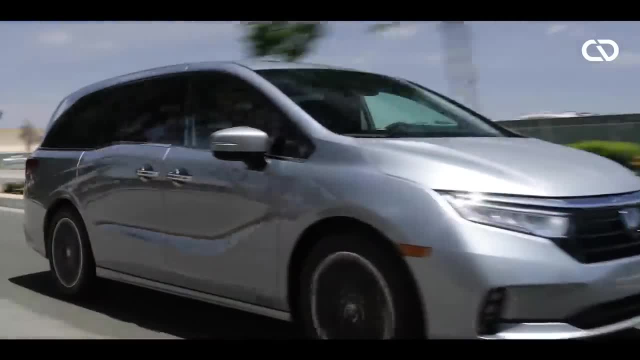 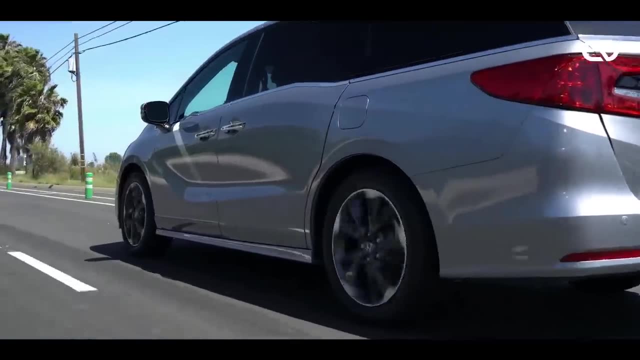 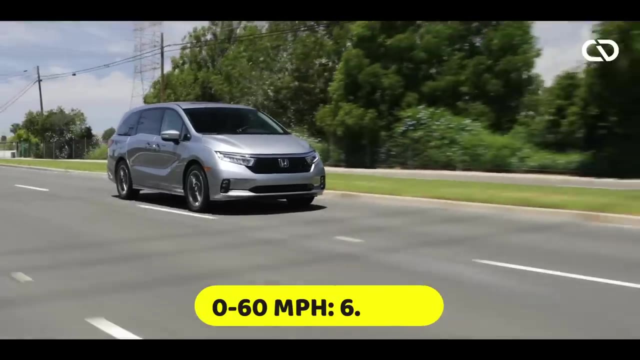 a very reliable engine, but it also produces plenty of power too, with around 280 horsepower and 262 pound-feet of torque. The transmission duties are taken care of by a 10-speed automatic and front-wheel drive system. The Odyssey is also quick on its feet: It takes only 6.6 seconds to 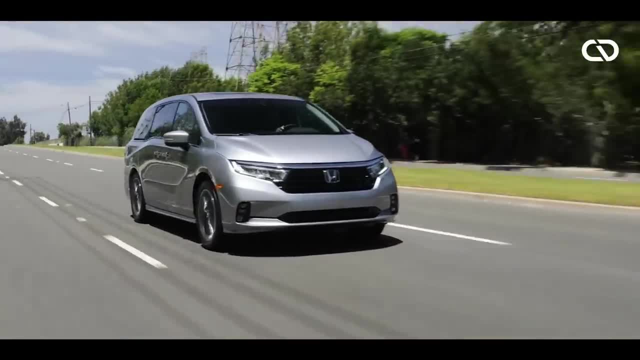 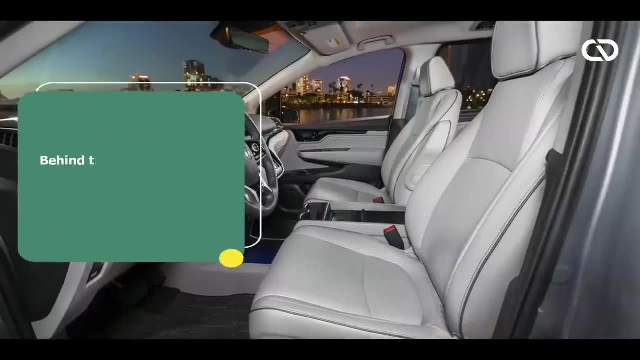 hit 60 miles per hour. Additionally, the Odyssey offers a great driving experience, which is also with a solid ride, comfortable suspension and good handling as well. The interior is spacious and made of quality materials and has lots of storage space. The Odyssey also offers a choice. 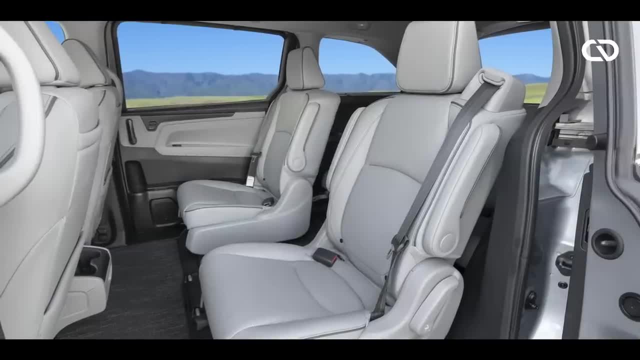 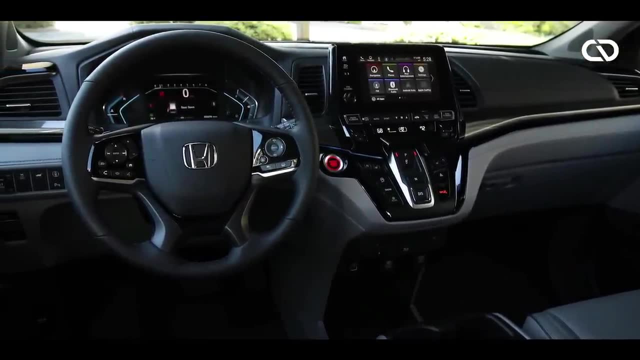 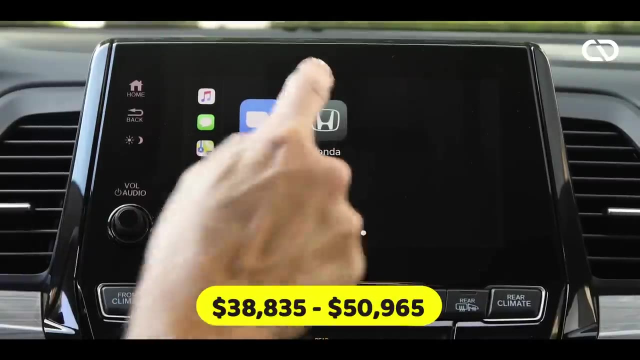 of either a 7 or 8-seats configuration, which you can choose depending on your needs. All Odyssey model gets an 8.0-inch touchscreen display with Android Auto and Apple CarPlay, although the infotainment display is quite dated. The 2023 Honda Odyssey comes with five different trim levels to 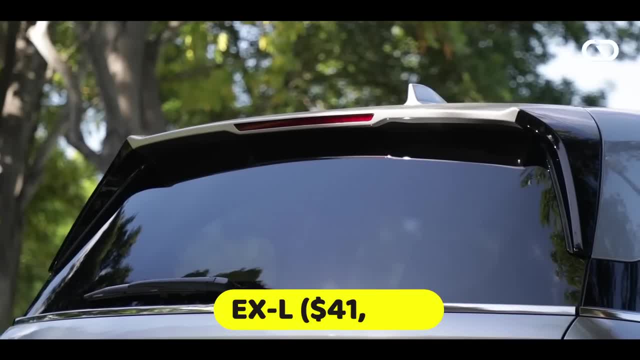 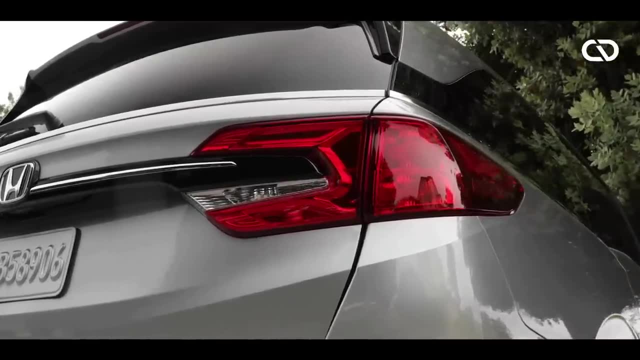 choose from, while the 2023 Honda Odyssey comes with a 5.0-inch touchscreen display, which is also a 5.0-inch touchscreen display, While we recommend the mid-range trim, the XL, which features leather upholstery, a moonroof and a power tailgate as well, These extra features are ones your family. 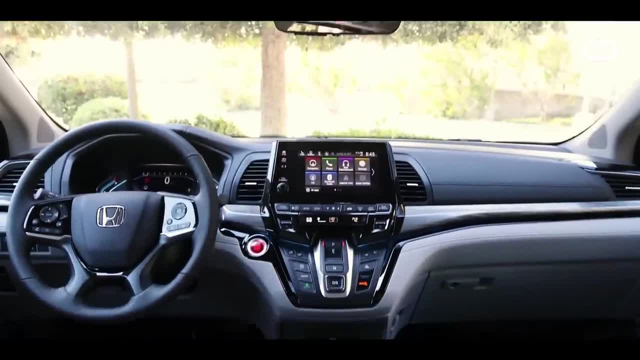 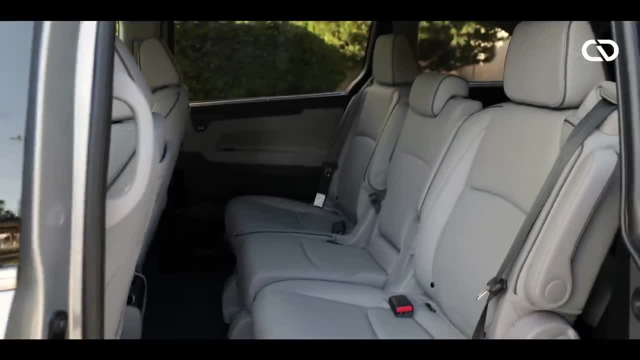 will love. In terms of safety features, the Odyssey features all the latest features you could want in a minivan, including standard automatic emergency braking, adaptive cruise control and blind spot monitoring. And yes, the Odyssey earns a five-star overall safety rating from the National Highway. 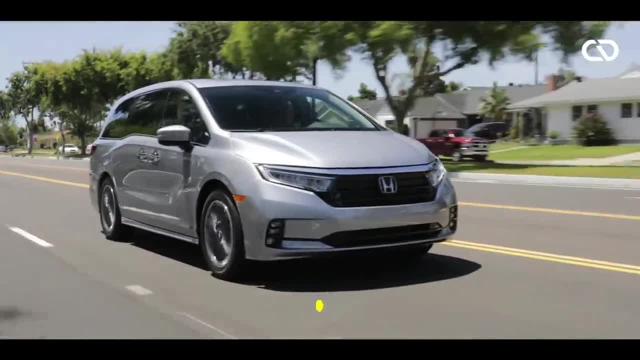 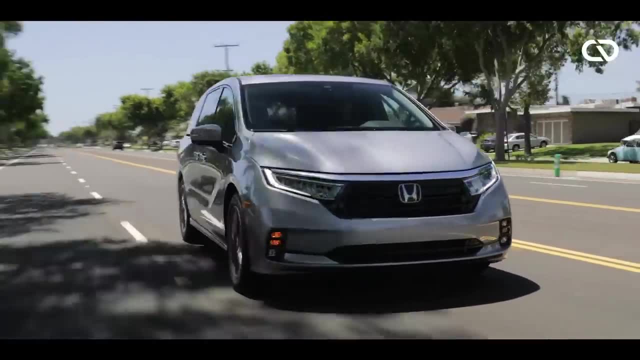 Traffic Safety Administration. The towing capacity of the Odyssey is up to 5.0-inch and the capacity is good: It can tow up to 3,500 pounds. With that said, though, the Odyssey does have a few downsides, such as the fuel economy is not impressive. According to the EPA, it can deliver. 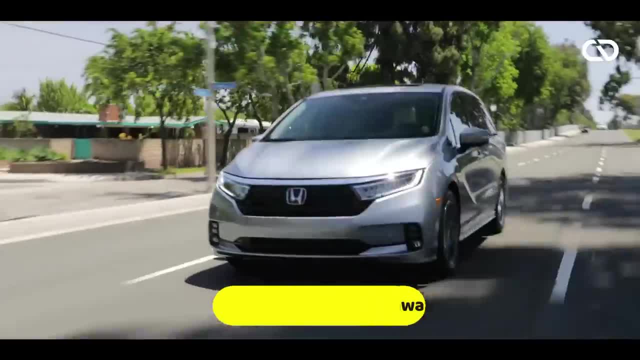 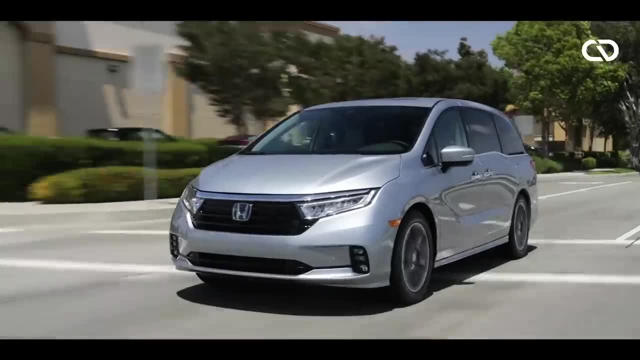 19 miles per gallon in the city and 28 miles per gallon on the highway. And, like the Carnival, you can only get Odyssey with the front-wheel drive, which is another drawback. So what's a car shopper to do? Well, look no further than the top pick on our list, which is the 2023 Toyota. 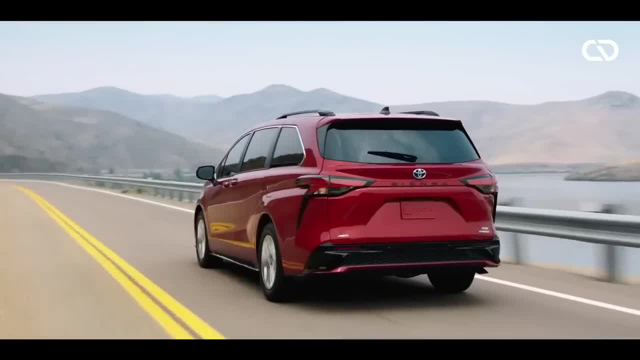 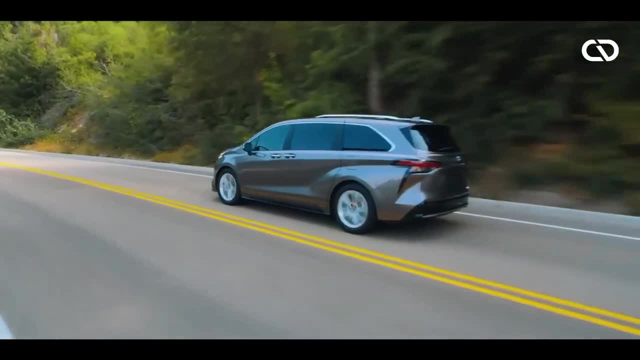 Sienna. The Toyota Sienna takes the top spot for the best minivan, with its long-term reliability, rugged exterior design, excellent fuel economy and top-notch safety features. Toyota has added a special limited edition to celebrate Sienna's 25th anniversary. 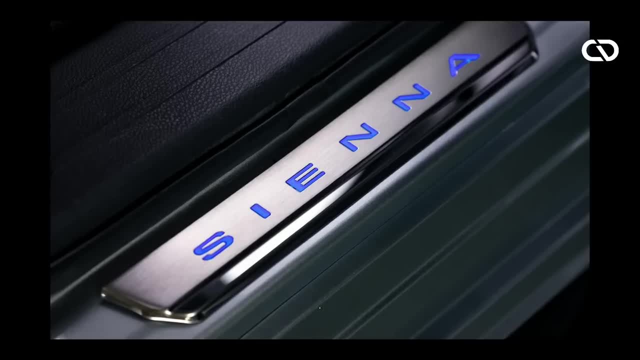 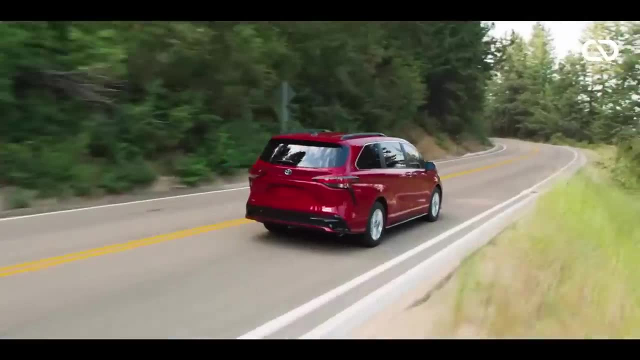 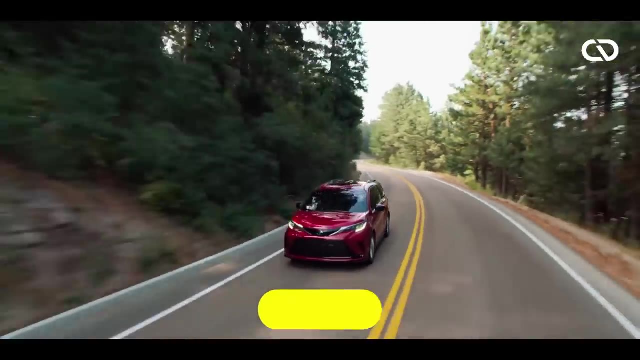 and only 2,525 units of them will be produced and will be based on the stylish XSE trim. However, we recommend buyers should stick to the most popular mid-range XLE trim as the best value for money, Because it starts at around $42,500 and offers a simple 2.5-liter four-cylinder engine paired. 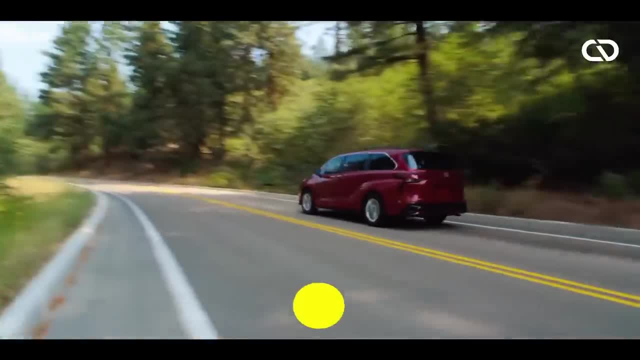 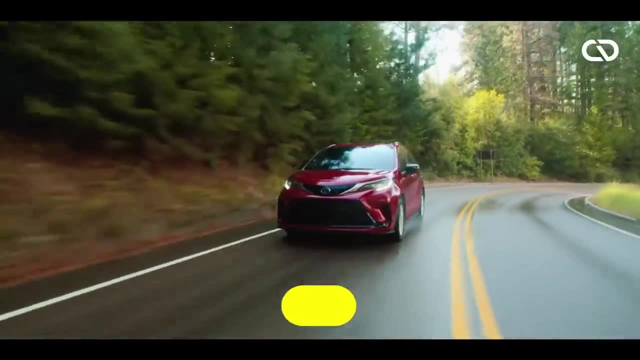 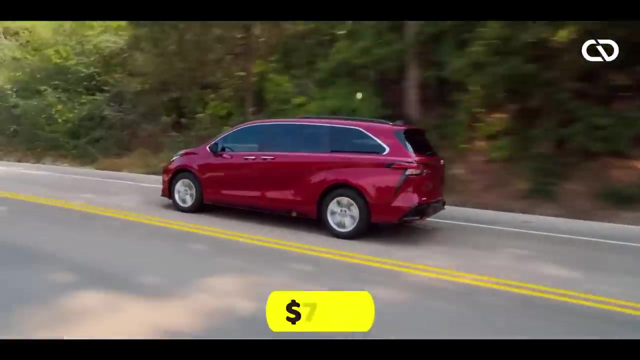 with an electric motor which produces a combined output of 245 horsepower. that's enough power to navigate easily through any traffic scenario. All 2023 Sienna trims come with standard front-wheel drive, while all-wheel drive can be added simply by paying an extra $760, which seems to be a 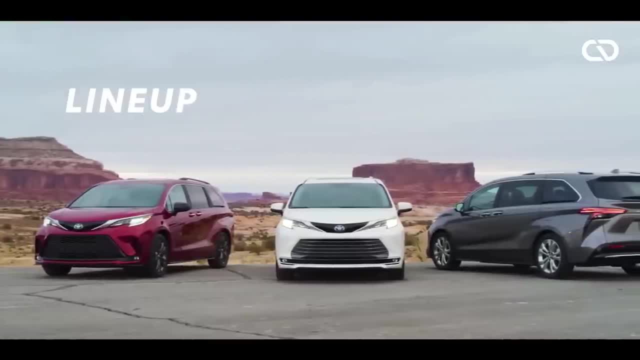 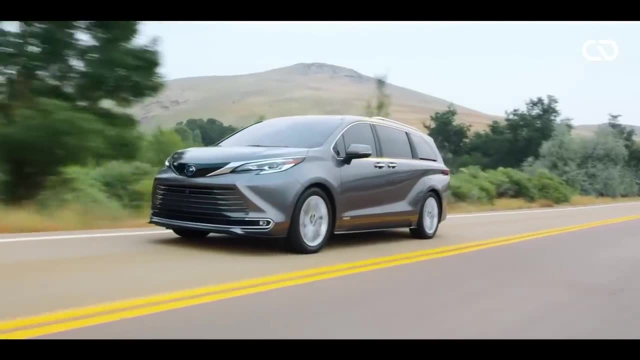 upgrade And, according to EPA estimates, the Sienna will deliver an impressive 36 MPG in the city and 36 MPG on the highway with a front-wheel drive system, And it has only one mile less with the all-wheel drive system, which is not even close. 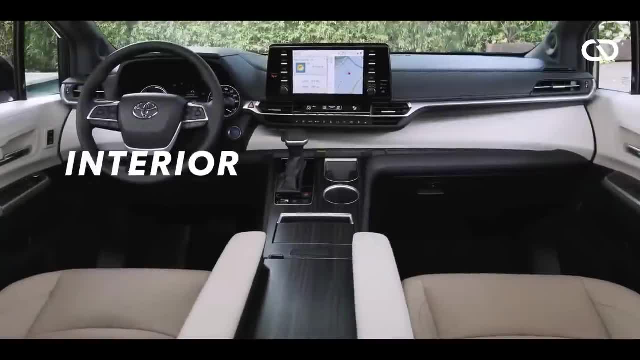 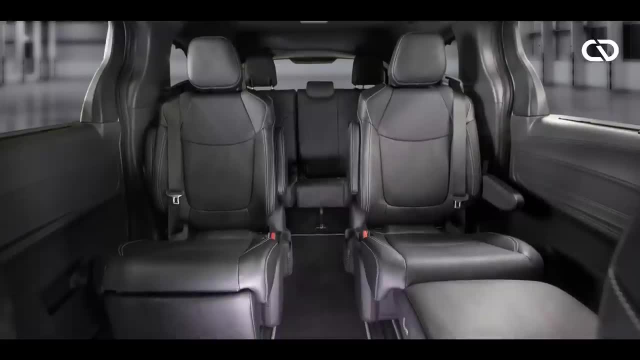 to any rival. The Sienna's interior is well-equipped and all trims offer standard eight-passenger seats, while a seven-passenger seat layout is also available, and optional second-row captain's chairs will make your long journey more comfortable. The minimalist dashboard comes with a standard 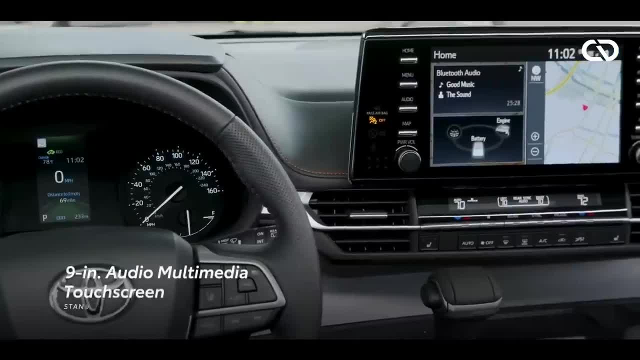 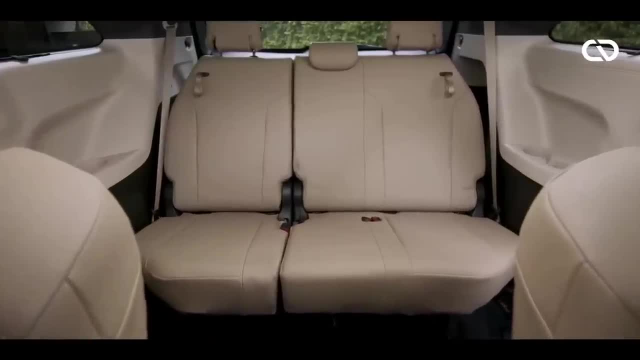 9.0-liter four-cylinder engine, which is a great addition to the Sienna. The Sienna's interior is a standard 6.0-inch infotainment touchscreen with Android Auto and Apple CarPlay, while our recommended trim, the XLE, offers synthetic leather, upholstery, multi-zone automatic climate control. 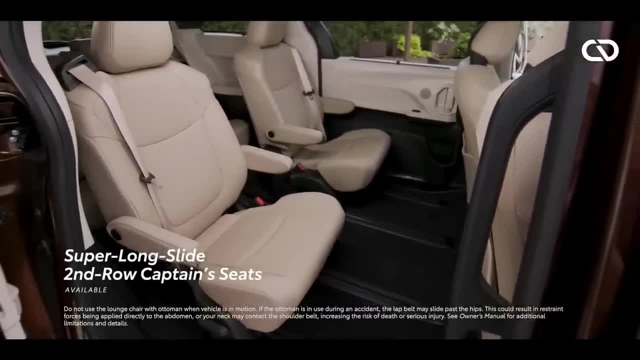 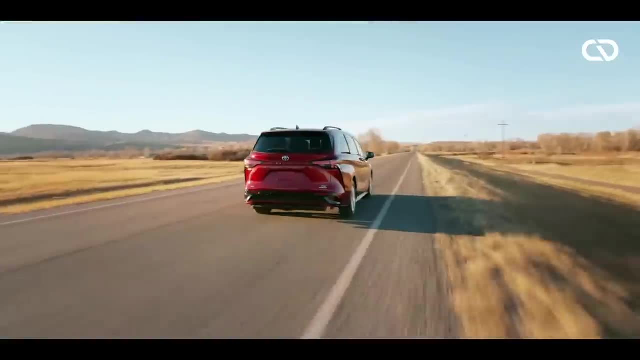 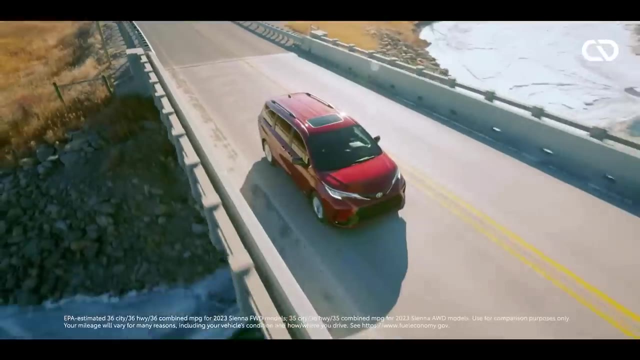 and heated front seats as well. Plus, the Sienna has the same 3,500-pound towing capacity. When it comes to the safety features, well, the Sienna comes with Toyota's latest Safety Sense 3.0, which includes all the latest safety features and driver assistance technology. 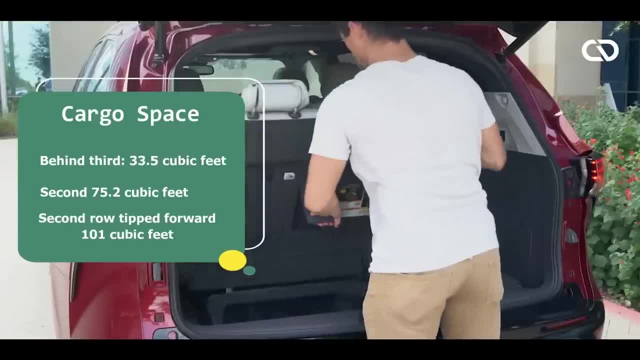 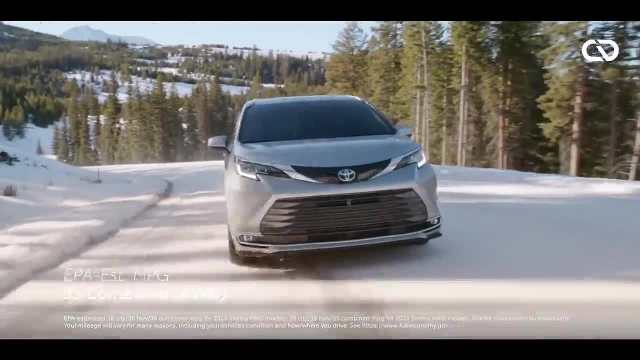 However, you can't remove the Sienna's second-row seats, which is a downside for some consumers. Despite this, for those who are looking for great fuel efficiency, long-term reliability and sky-high resale value, the Toyota Sienna is definitely worth considering.